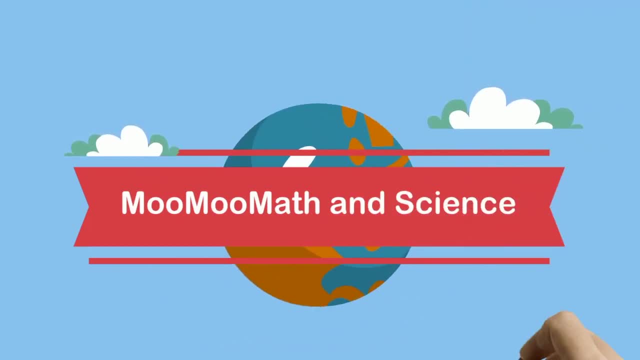 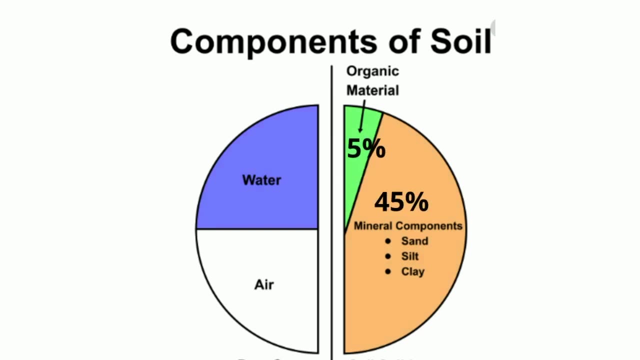 Welcome to MooMooMath and Science and Soil. If you look at a chart of soil, you'll see that it is made up of 45% minerals, 5% organic matter like decaying plants and animals, 25% water. 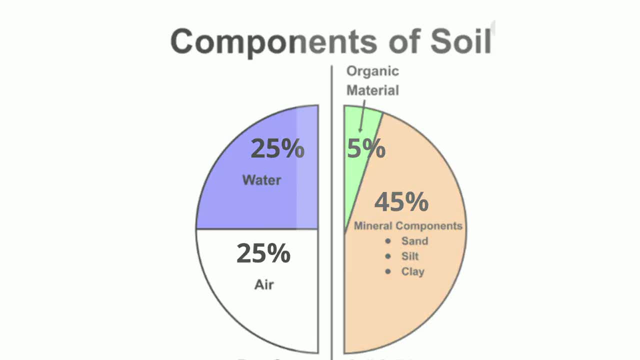 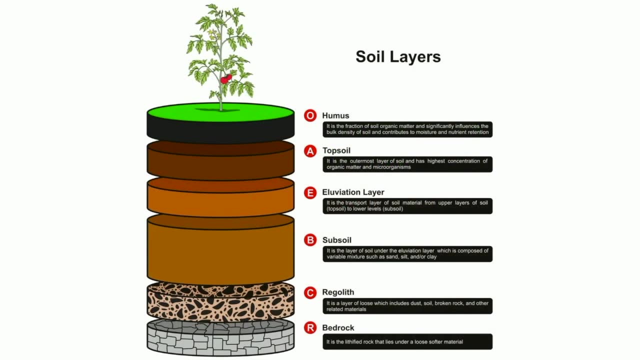 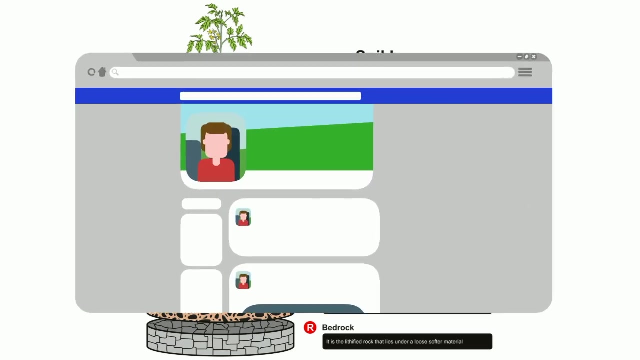 and 25% air. You can also study soil by looking at its profile and the soil horizon. A vertical layer of soil that shows all of the different layers is the soil profile. Much like your profile on Facebook, it tells others all about you. The profile of the soil. 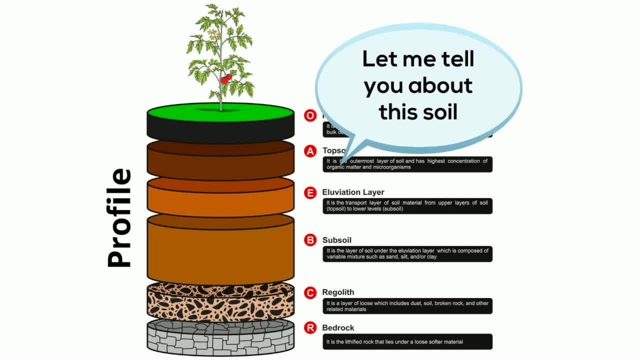 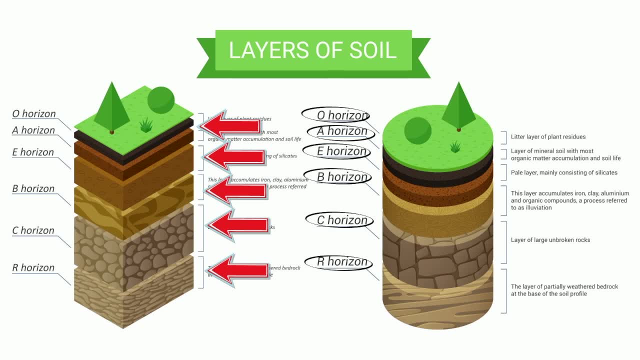 tells all about the soil. A soil horizon is each individual layer of the profile. Each layer has different physical properties. The horizon layers are O, A, E, B, C, R. Let's take a look at what each layer is made up of. 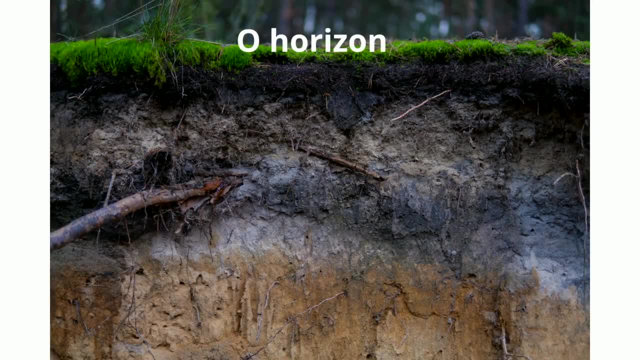 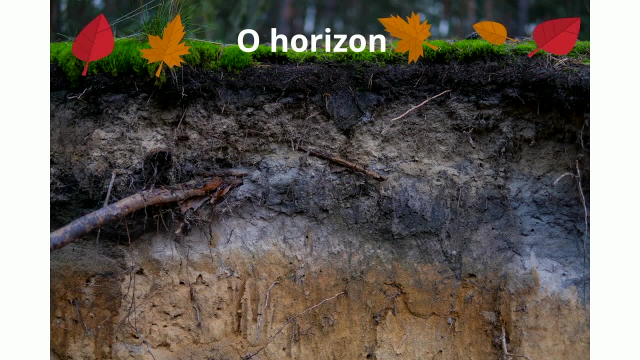 The O layer, or horizon, is also called the litter. It's composed and contains dead leaves, twigs, sticks, fallen trees. The O horizon is thin in some soils, thick in others and not present at all in some types. 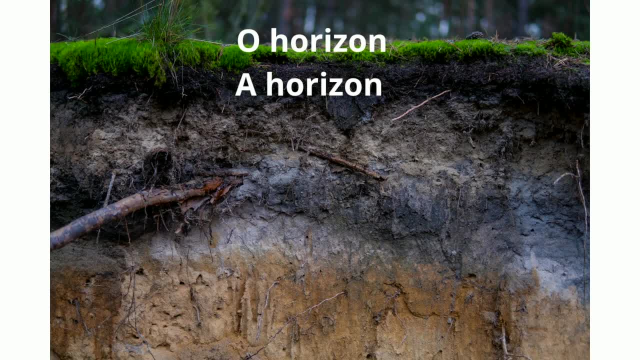 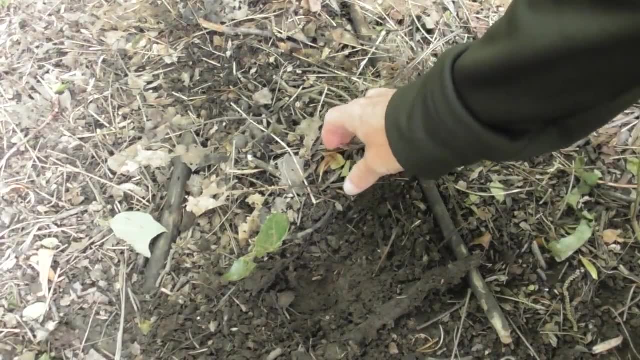 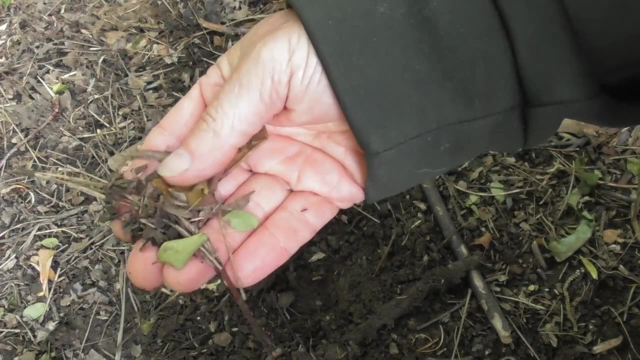 The A horizon is also called the topsoil. It contains rich organic matter, along with some minerals. Ok, let's see the difference between the litter and the topsal a. The litter you can see is composed of twigs, leaves. 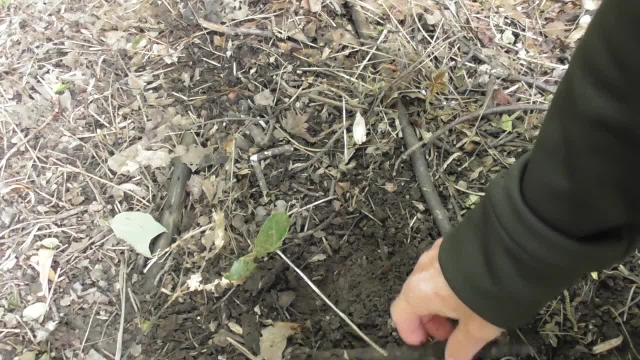 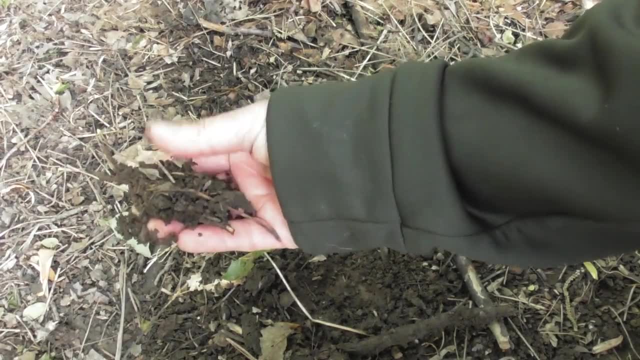 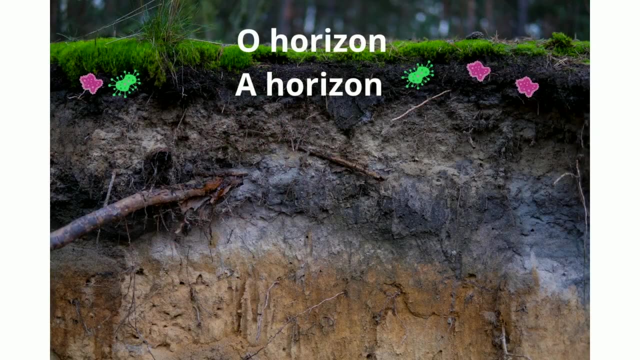 okay, Then what happens is you get decomposers. You get worms, bugs, etc. Wow, and it creates this, as everything decomposes this: really deep, rich, full of organic matter, topsoil. The remains of these plants and animals create a mixture called humus. 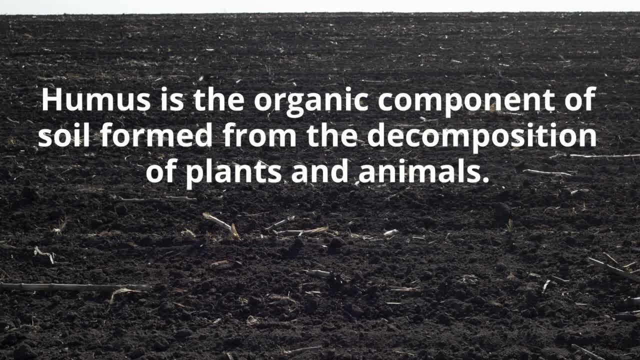 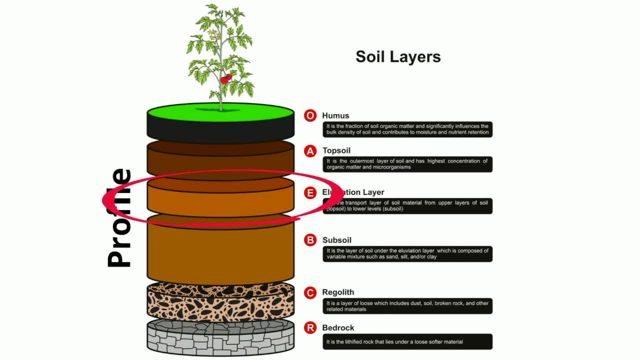 which is dark organic material that forms in soil when plant and animal matter decays. E is also called the alluviated layer. As water moves down the soil, substances are removed and pulled out in this layer, resulting in a concentration of sand and silt particles.